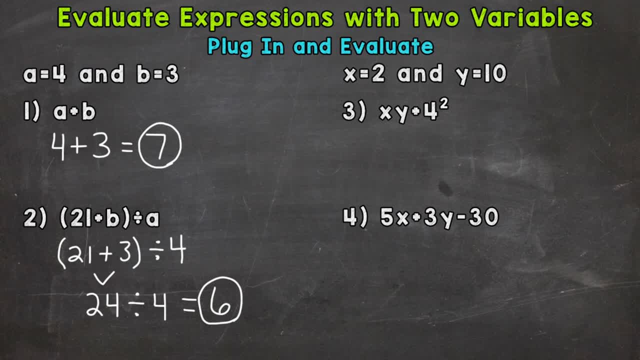 to a letter. it's going to be multiplication, So let's plug in and evaluate. So x is going to be 2 times y, which is 10 plus 4 squared. Now we need to go through our order of operations. So any parentheses: No, Any exponents: Yes, So. 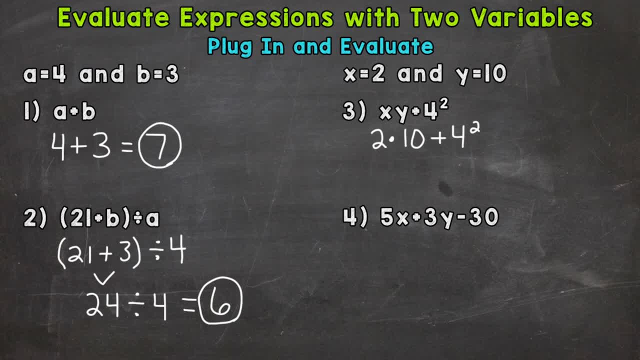 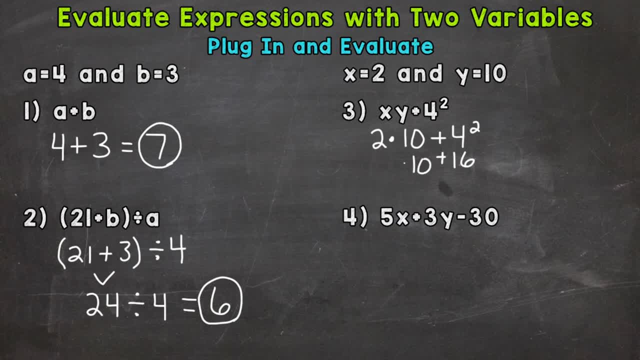 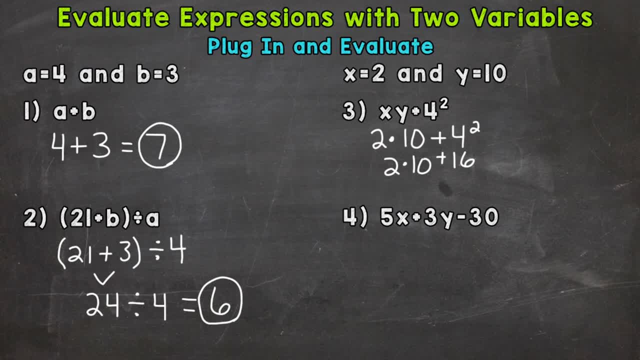 multiplication or division. yes, so that's what we do. next, we have 2 times 10, which is 20. bring down our addition and the 16, and that's where we end. so 20 plus 16 equals 36. and lastly, number 4. we have 5x plus 3y minus 30. now, remember whenever. 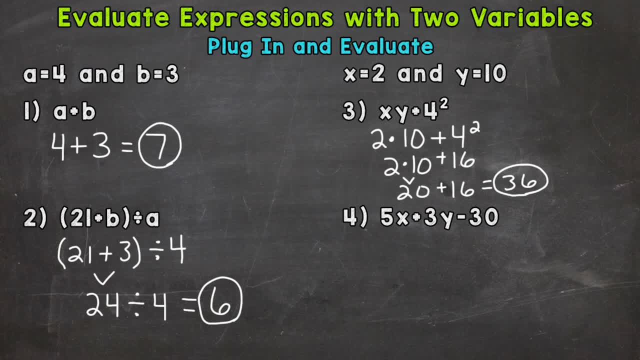 you have a number next to a letter or a letter next to a letter. that means multiply. so plug in 5 times 2 plus 3 times 10 minus 30. so we plugged in together and we have 36 plus 3y minus 30. so that's where we end, so we plug in. 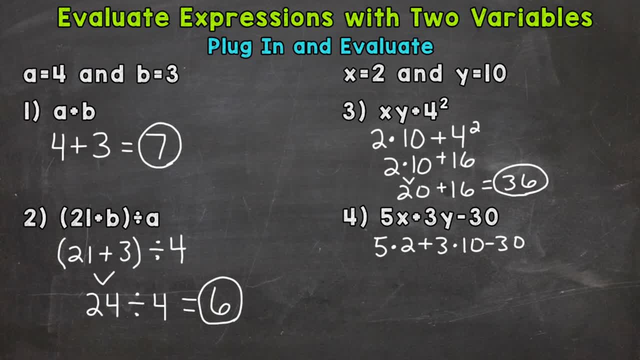 together. and we have 36 plus 3y minus 30, so we plug in together. and we have 36 plus 3y minus 30, so we plug in. so any parentheses, no, any exponents, no, any multiplication or division. yes, so that's where we start. now we have two multiplication problems, so we can work. 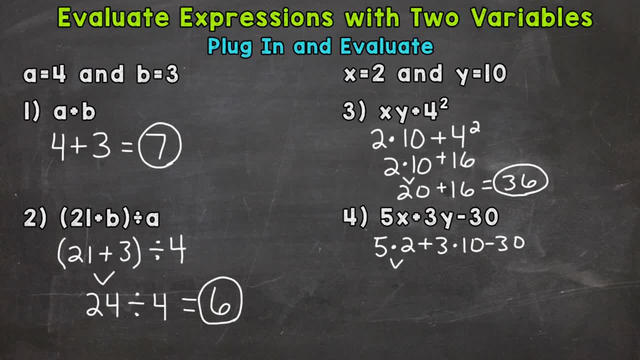 our way from left to right. five times two is ten, and we'll bring down everything we do not use. and now we can do the other multiplication problem. three times ten is 30. bring down everything else in the same exact order, and now we have addition and subtraction. 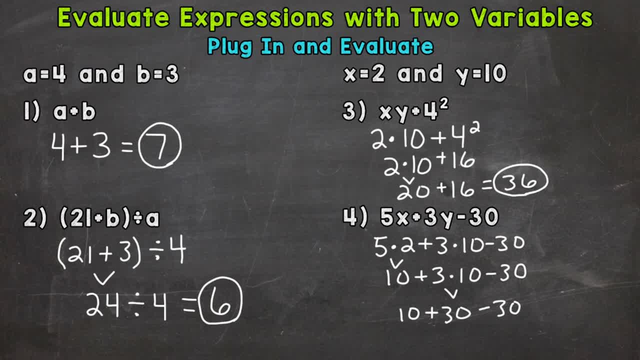 now addition and subtraction are in the same level, so to speak, of the order of operations, so we can work our way from left to right. so let's do addition: 10 plus 30 is going to give us 40. bring down our subtraction and the 30 and that's where we will end: 40 minus 30, which gives us 10. 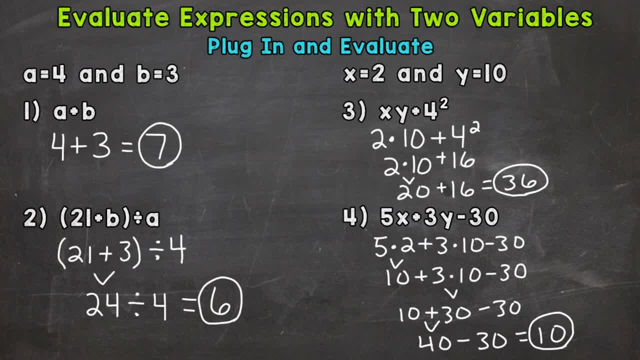 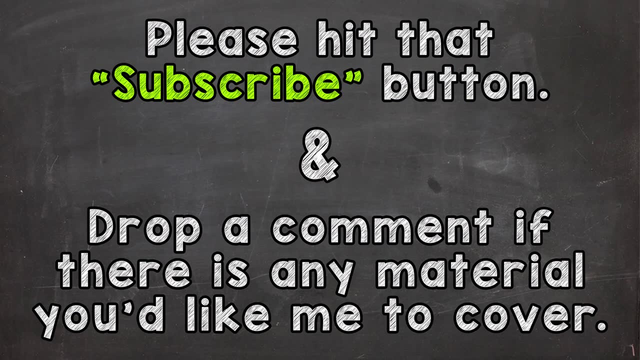 so there you have it. there's how you evaluate expressions with two variables: plug in and use the order of operations to evaluate. i hope that helped. thanks so much for watching. until next time, peace you. 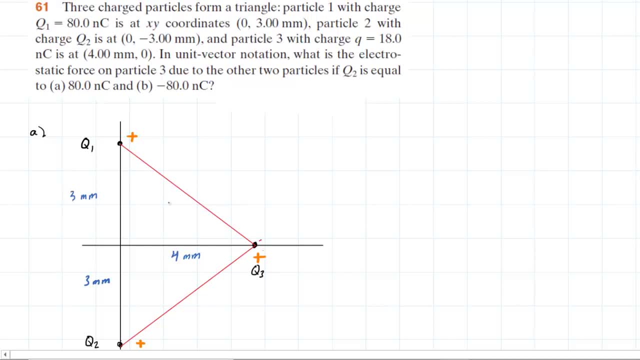 In part A of the question we are told that the particle Q2 has a positive charge on it. so we have indicated that positive sign right there for the charge Q2.. We've also drawn the rest of the configuration based on the given information. 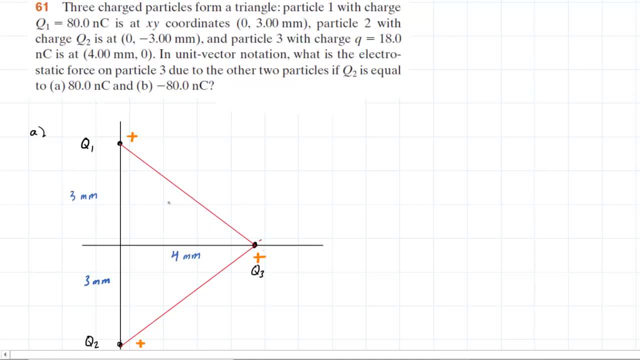 One thing we will need is the distance from Q1 to Q3, as well as the distance from Q2 to Q3, although we can see that those distances will be the same. So, in other words, we're going to need this distance right here. We're going to call it R.